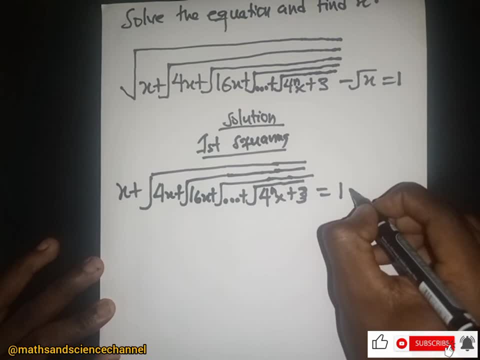 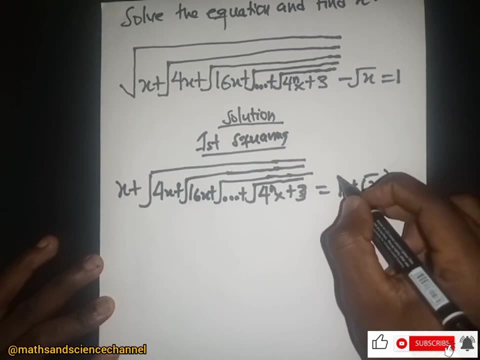 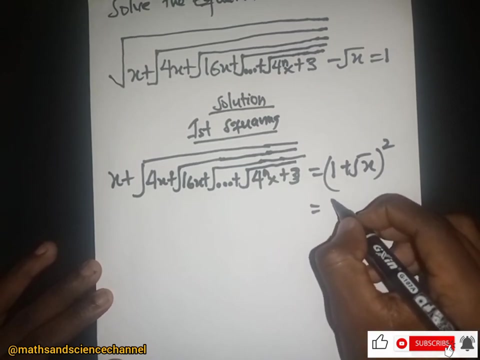 Then being equal to 1 here. So let's send this to the other side, plus square root of x. So we have also squared that. So, squaring that we just have, we are going to get the whole of this to be So 1.. 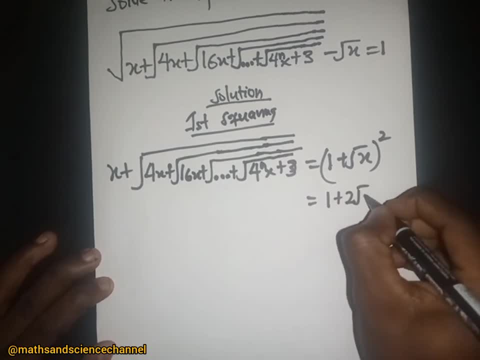 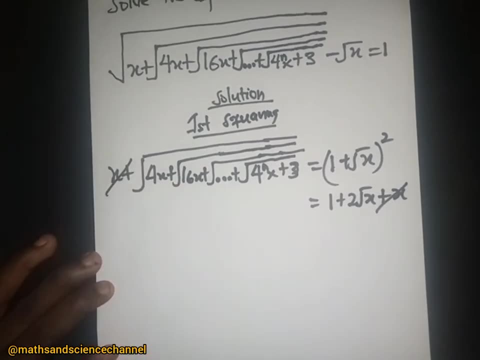 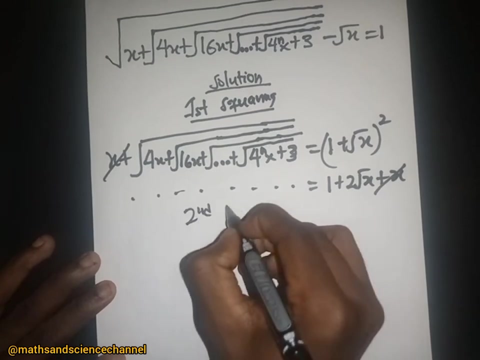 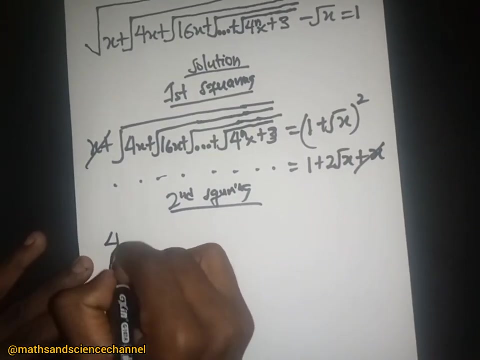 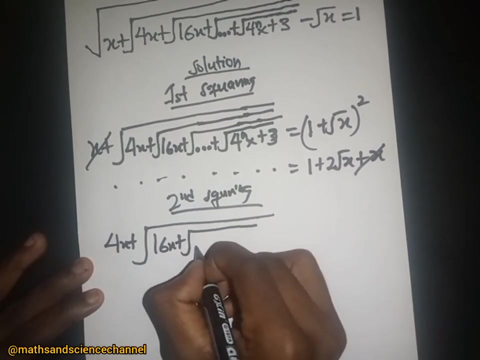 So when we expand that, we just get 1 plus 2 of the x, Then also Plus x. But you realize that this will get rid of that, right? So in this case we just repeat the whole thing. So this is what we have Now. we do the second squaring, We square again. So we square for the second time, So, squaring for the second time, we have 4x plus outside, Then we have 16x plus. That goes all the way. 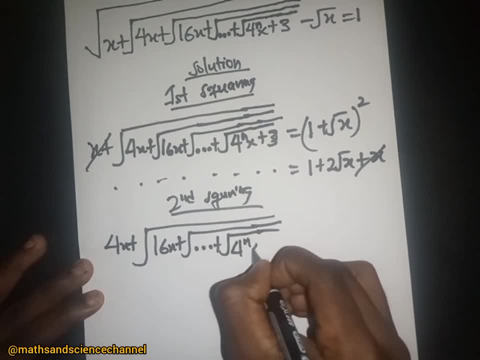 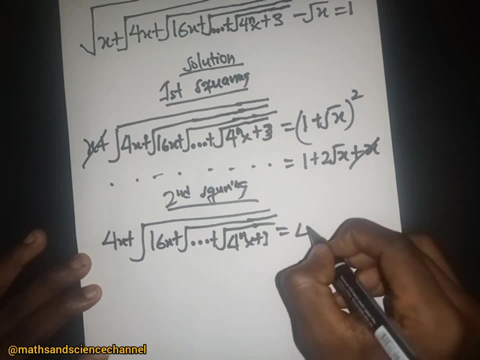 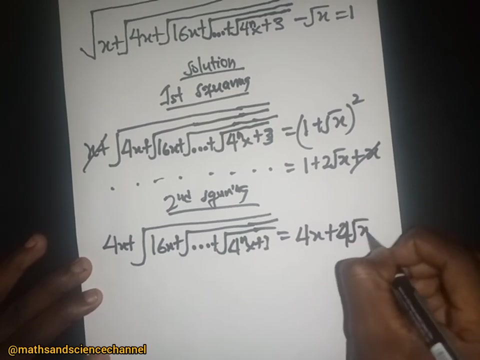 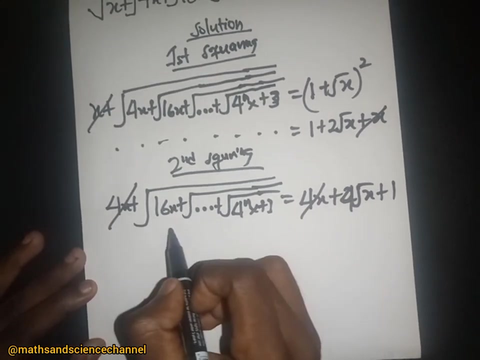 Then we have 4 power x plus 3 here. Then we square again Now when we square this side, So when we square with this side, we are just going to get 4x here, Then plus 2.. Sorry, 4 root x, Then also plus 1.. So this will also get rid of that for the second squaring. So we will continue to do it for the rest and it will continue. 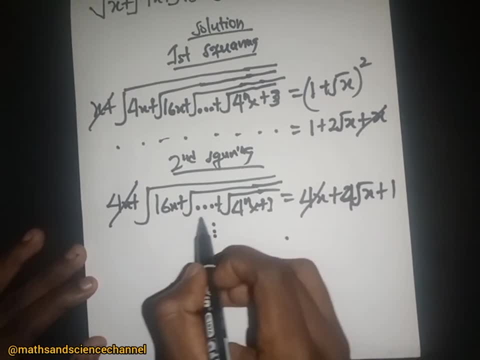 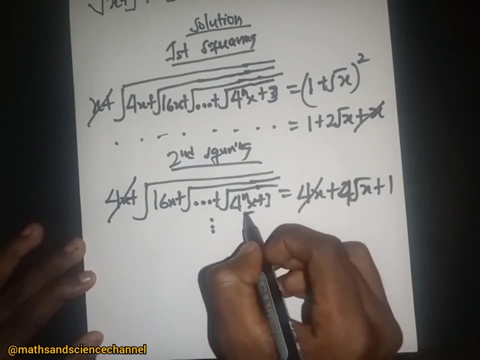 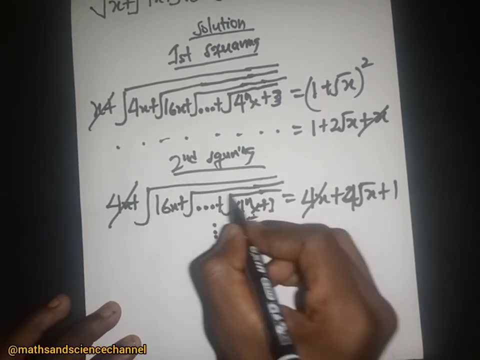 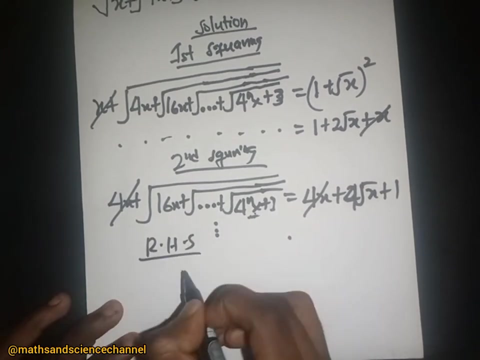 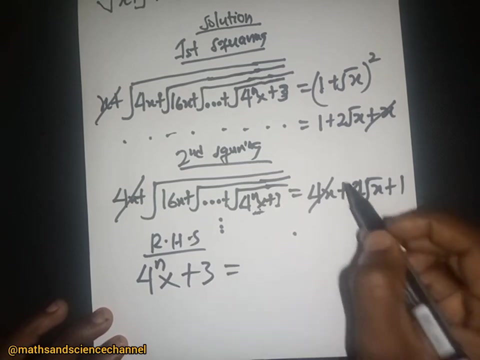 So we can do it for the rest continuously. So we can do it for the rest of this dot all the way to that. But you realize that in doing this we are just going to leverage. So after getting rid of the squares continuously and we get to the last part, we are only going to get for the right hand side. So for the right hand side here we are just going to get 4 power and then x plus 3, here being equal to 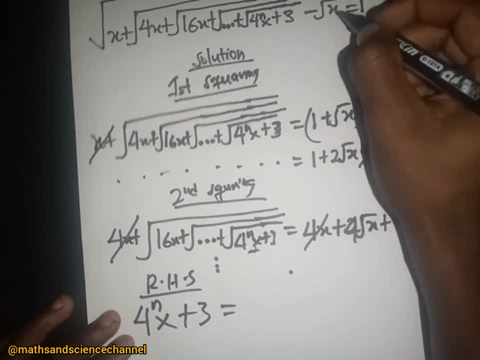 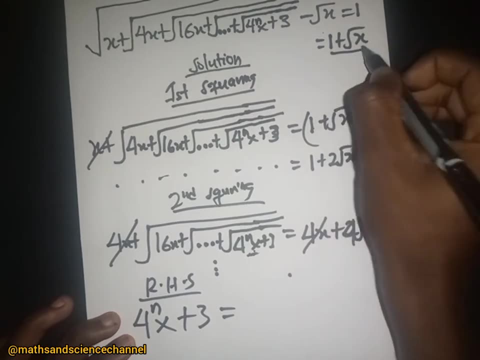 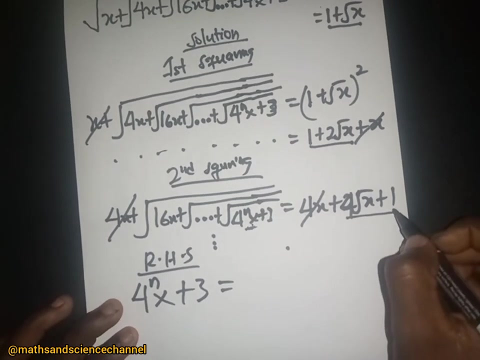 Now, if you look at the right hand side, we started with- So let's write this this way, So we have 1 plus square root of x, and we came to, So we had this, The next thing, we had that, and we also had this, So we realize that the last part, here we are just having the square root of x plus 1 throughout. 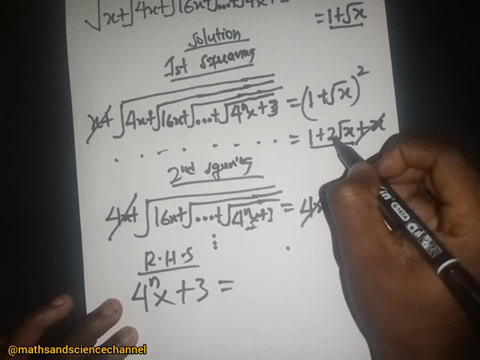 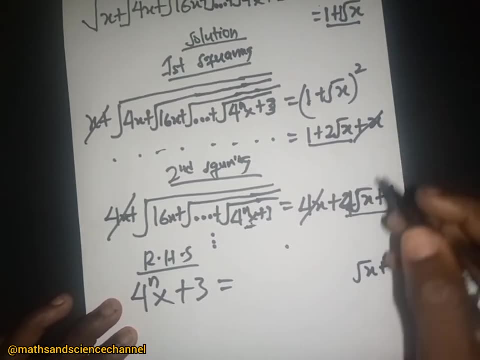 But then also we have 2.. We have 2.. We have 4.. Sorry, we have 2 and also we have 1 here Continuously. So it's just like a sequence, right, But it will follow in the squares of 2.. So we have 2 here, right, Then plus. 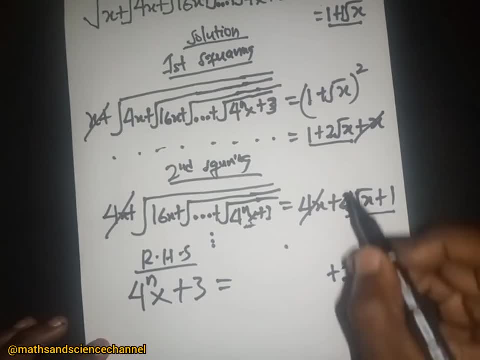 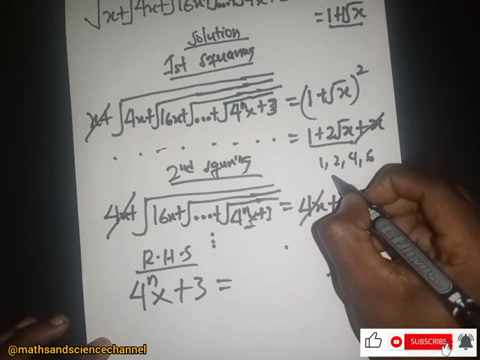 So it is moving between the series. So we have 1,, 2,, 4, 6 continuously right. So we can get an equation in this way: 2 to the power n multiplied by 2. So that when n is 1.. 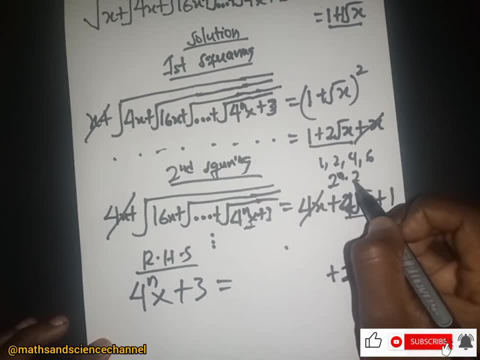 Starting from 0.. When n is 0, then we have 2, right. When n is 1,, then we have 4.. When n is 2, we have 4 here, Then we have 8. So continuously. 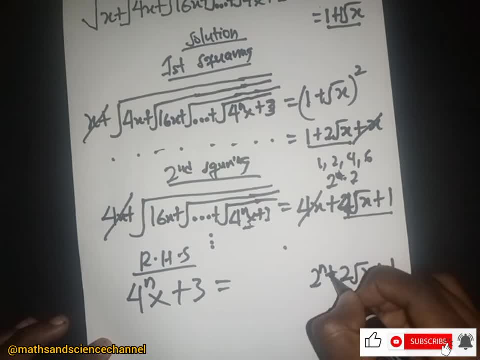 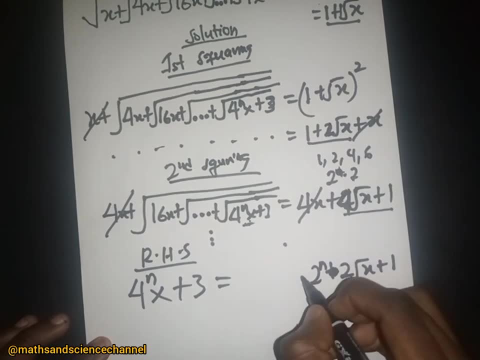 So we are going to have it in this way: 2 to the power n being multiplied by 2, right, That will be for these values over here, The series over there. Now we realize that we have 4x. We had 4x here. 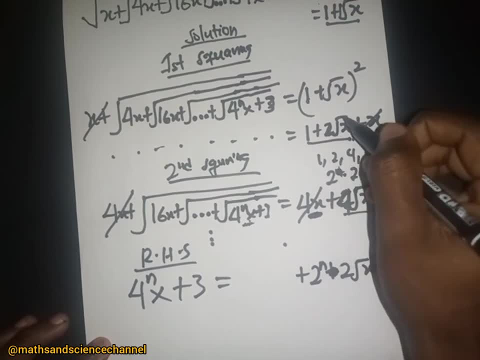 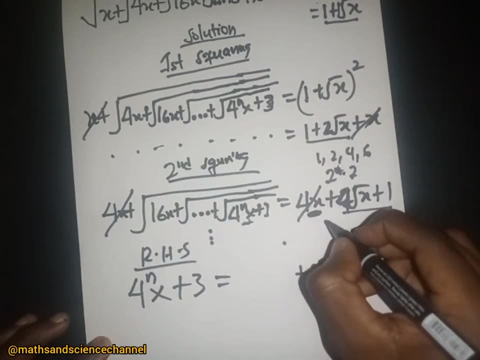 So in this case we also had 2x right. In the first case we just had x, which got rid of the x here. So in that case also we had x as the first term. Then we have 4x right. 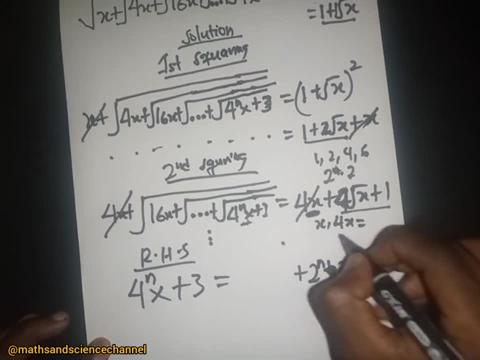 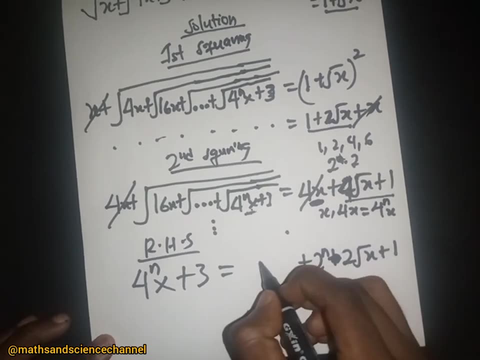 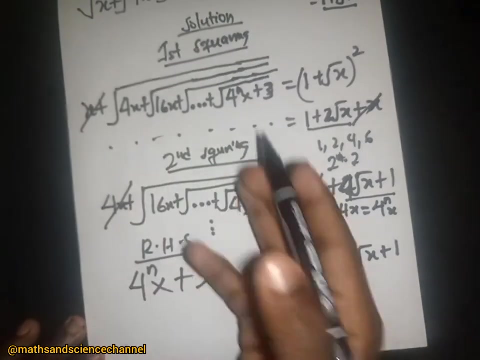 So we can also write an equation for this which is just going to be 4x here, Then in the series of n right. So we are going to have 4x here, then to the power n right. so this is what we have for the whole um equation over there. so 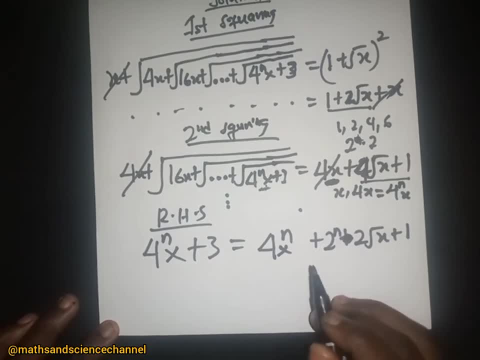 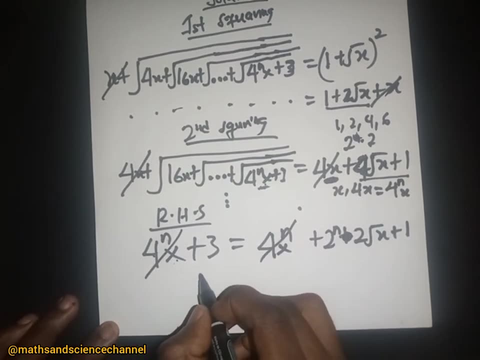 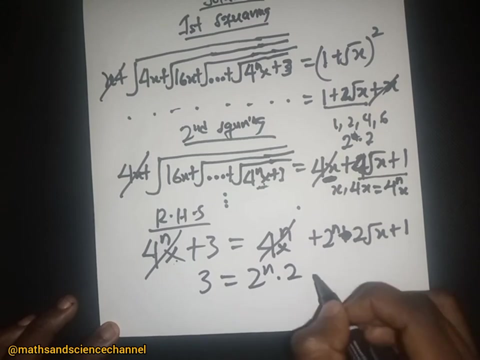 now the question is: you find the value of x right, you find the value of x. then you realize that 4 to the power n x. here we'll get rid of that and we are just left with um 3 here being equal to 2, power n multiplied by 2, then we have square root of x plus 1.